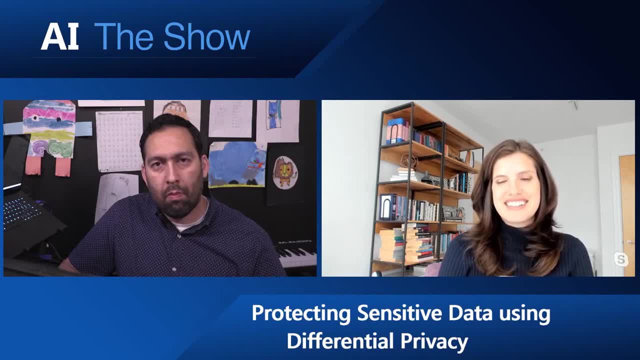 And I'm not sure I can think of a way to figure out which is which, and I'm not sure I can think of a way to figure out which is which, where I'm typing an email saying, basically you know, my social security number is and. 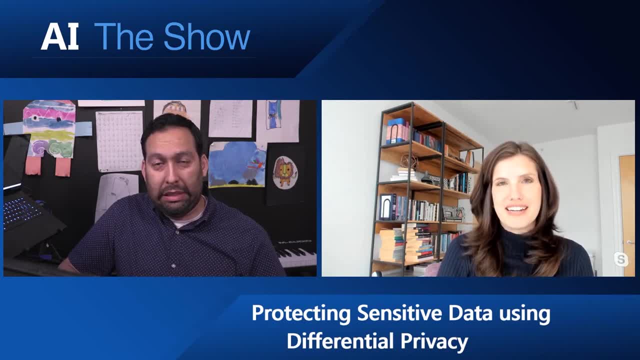 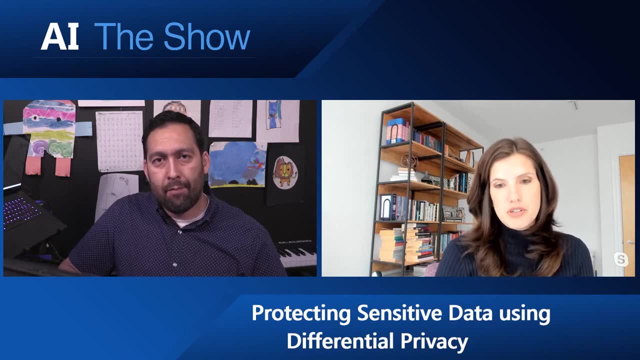 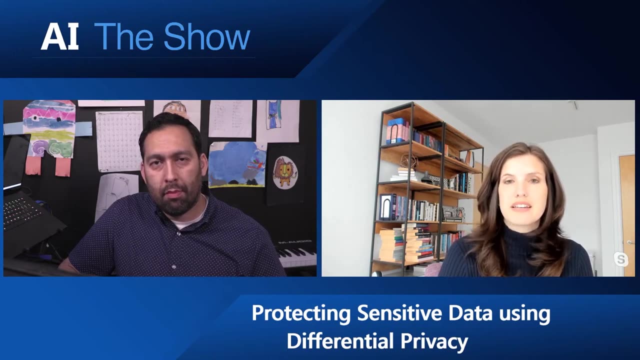 the model auto-completes with the social security number that it found in the data set, which would be a problem. And we can have the same sort of issue with statistics, where if you publish statistics or aggregate results from a data set, it's often possible to put those results back together. 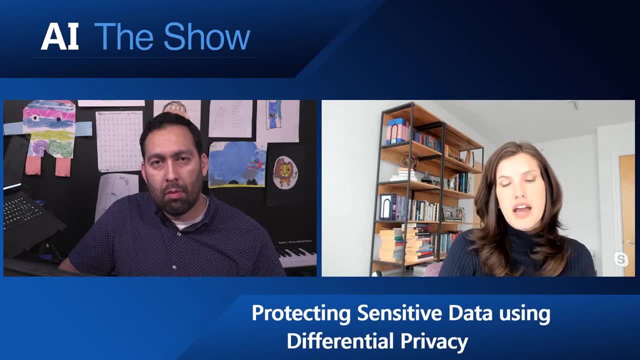 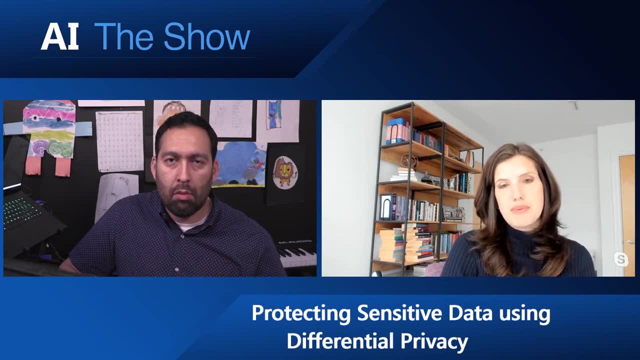 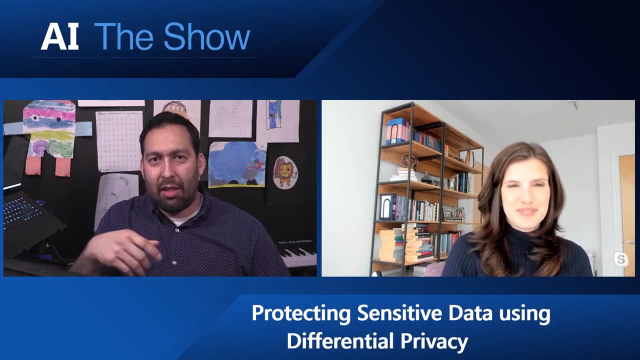 and actually recreate the underlying data set, And this has been used to find very sensitive information about individuals, based on public data sets, for example. So let's pause right there. What you're saying, then is, even if I'm only outputting the aggregation like, here's the: 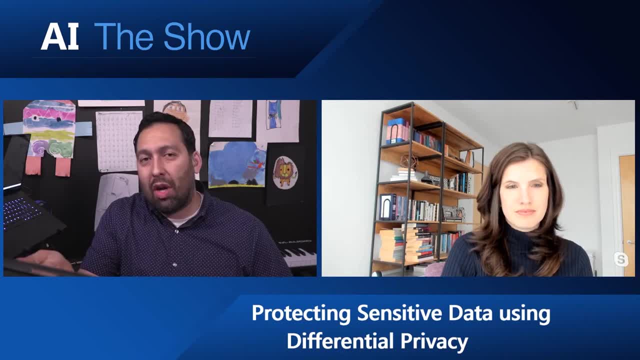 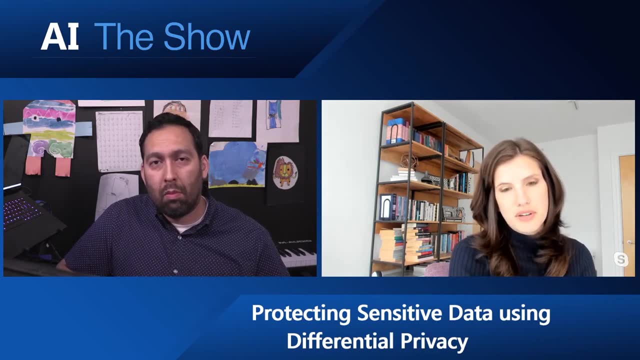 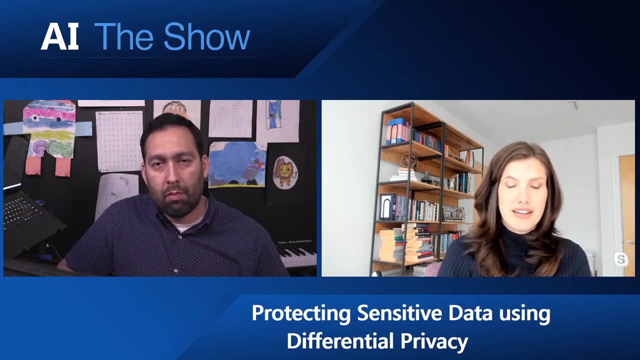 sum. here's the average. I can somehow reconstruct individual records, single items that are not in the aggregate. Yeah, absolutely So. it depends on how. It depends on how much information you have and how much computational power, but there's different types of attacks that, in fact, can be quite easy to do. that will reveal private 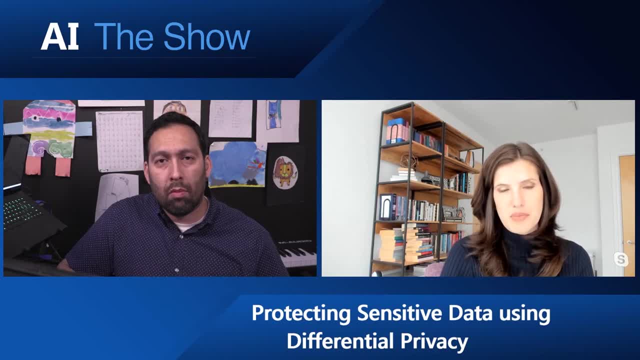 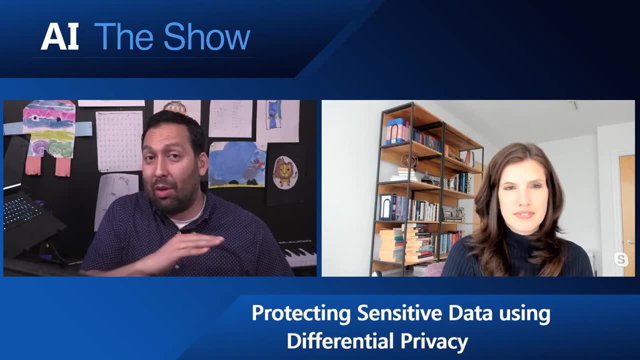 information, or at least give you a good guess at the private information. I'd love to see that because that's surprising to me, because most people try to obfuscate their data by only releasing aggregate data like average, whatever mean mode. 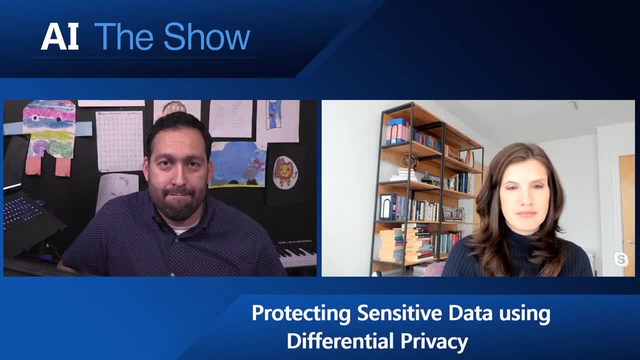 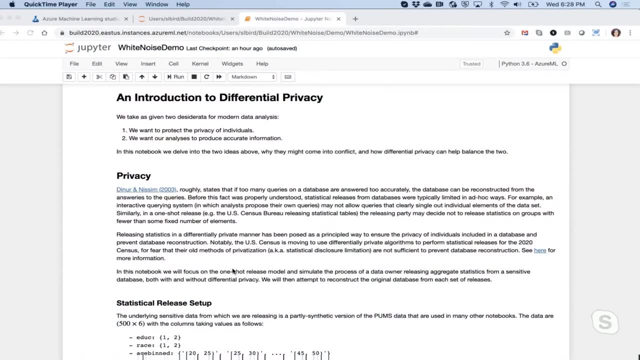 But you're saying you can actually reconstruct. I'd love to see an example of that. Sure, Let me show you. Let me show you an example in my notebook here. Great, So what I have here is an example. that is a synthetic example so that I can run it locally. 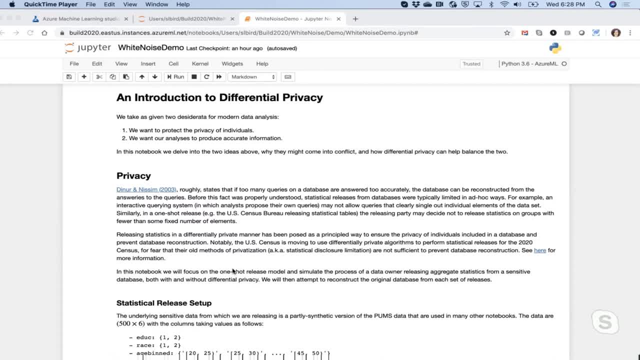 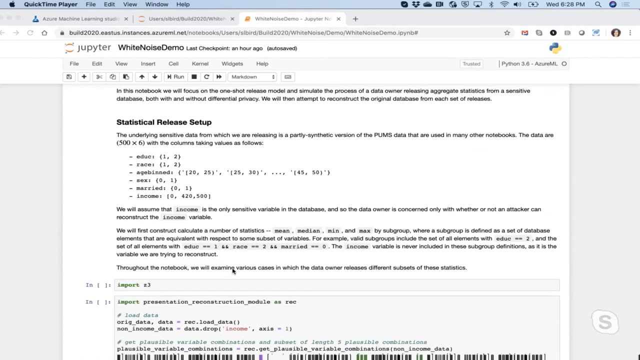 on my machine, but it's actually very similar to what the US Census demonstrated this past year as well. So it's taking a type of report that the Census releases and instead we're filling it with fake data. that's synthetic, Okay. 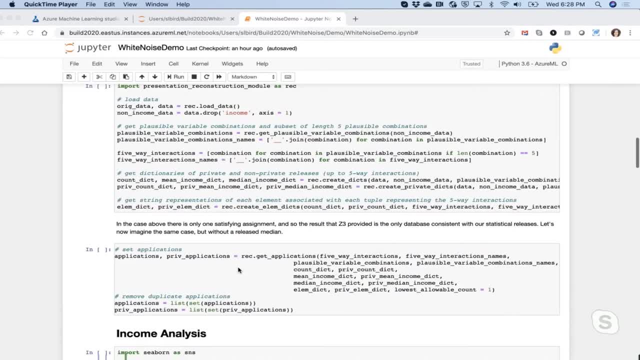 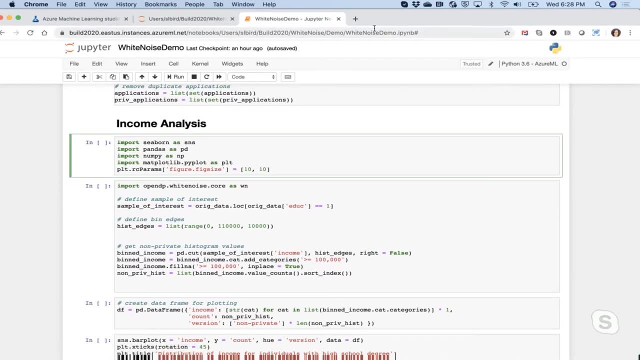 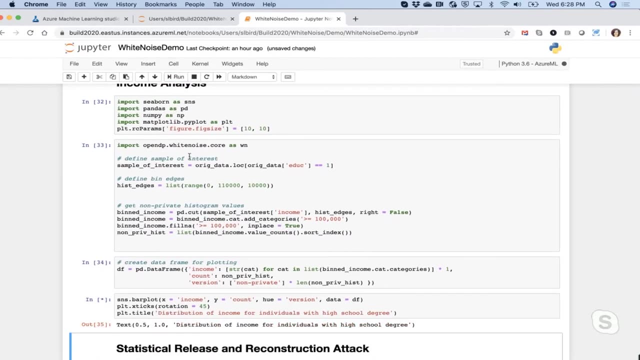 But it still holds the same, And so what I'm going to do then is I'm going to take this data, and what I'm trying to do is I want to do an income analysis. So what I'm going to do here is I'm going to run and I want to actually study the distribution of income for individuals with a high school degree. 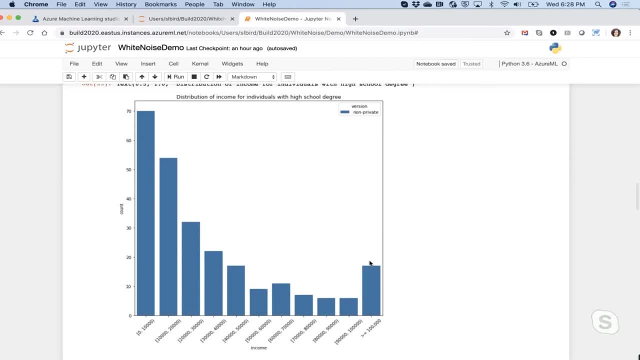 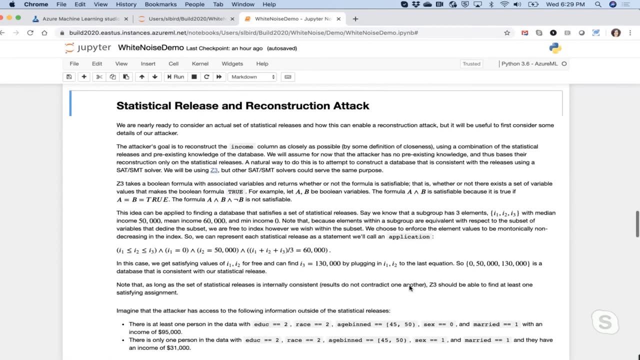 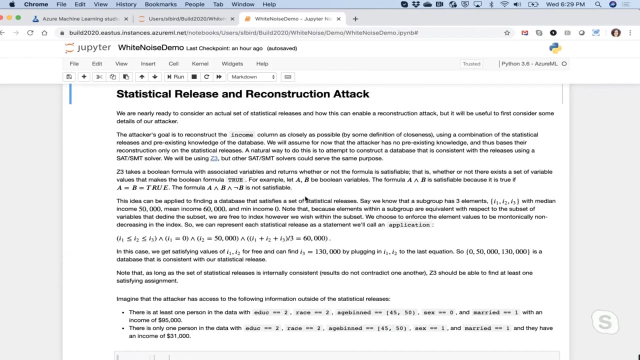 So I get a distribution here and you know, I can use this to do the analytics, Okay, Okay. However, the attack that I want to show you is what I've done. here is taken, a simple, off-the-shelf SAT solver that you can actually just- you know- pip install. 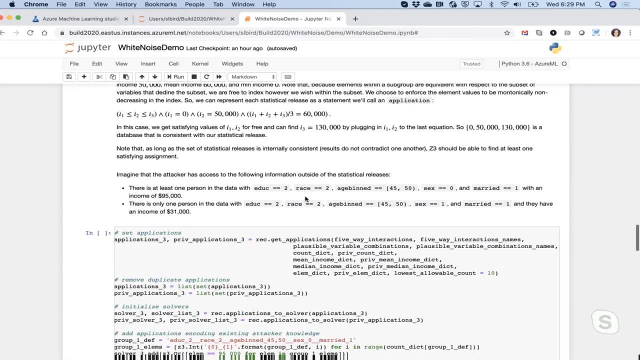 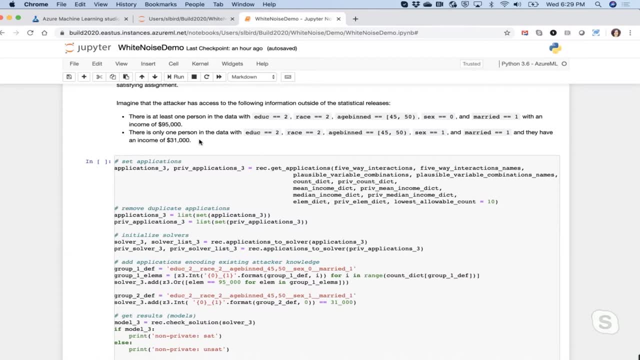 Anyone can use it And in this case I've assumed that I know just a little bit of information. I know very specific data points in my data set about a few people And what I'm trying to do is guess that income right. 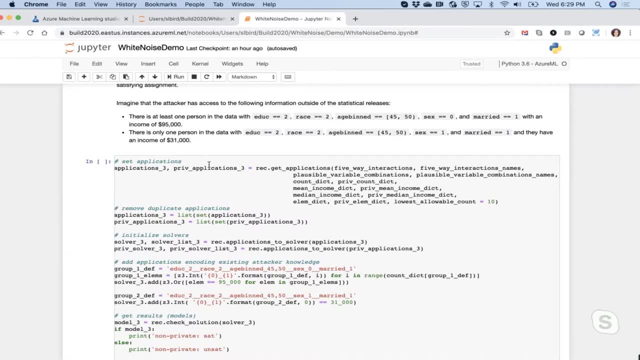 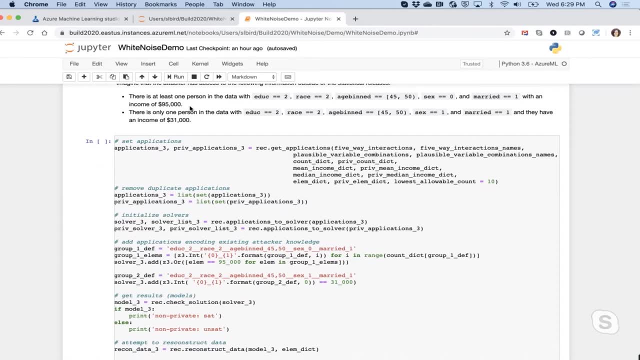 The income is the private, And so what I'm going to do is I'm going to let my SAT solver see if it can create a version of the database that matches up with the published results, the results that would have been in the census report. 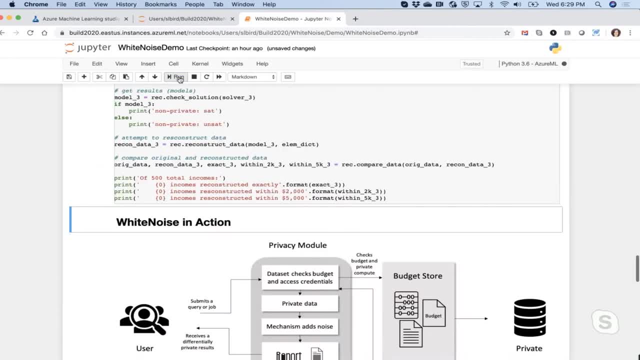 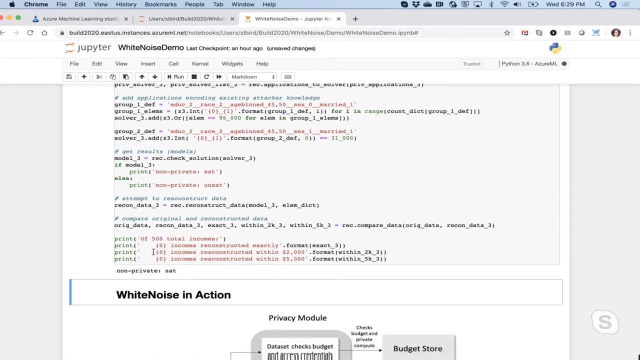 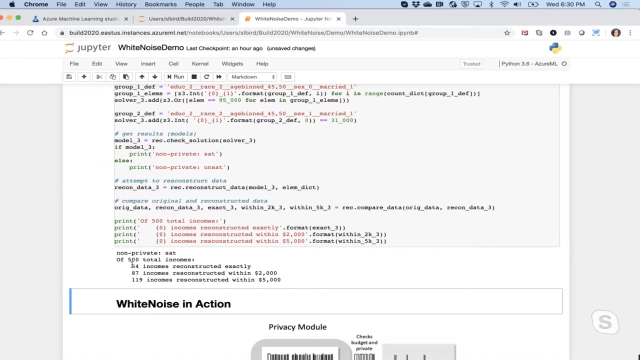 And so if we run here, I'm going to click down. So what we actually see is it's still running and trying to find an example And what we found is there's five, There's 500 individuals in this data set, But we were able to correctly guess the income of 50 individuals exactly. 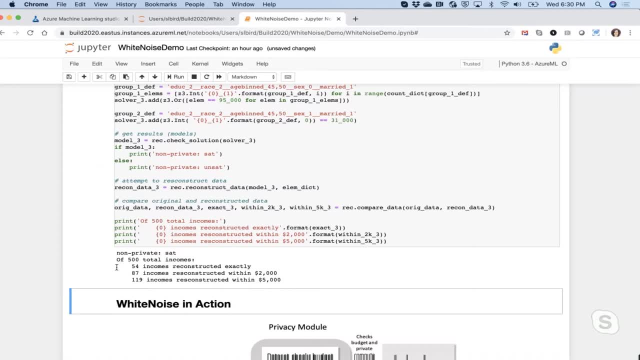 There were more than 80 individuals where we were guessing it within $2,000. And 120 individuals where we were guessing it correctly within $5,000.. Holy cow, So can we scroll up, Because I'm obviously not as smart as you. 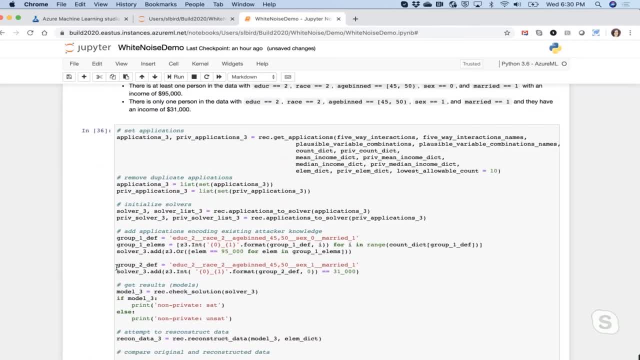 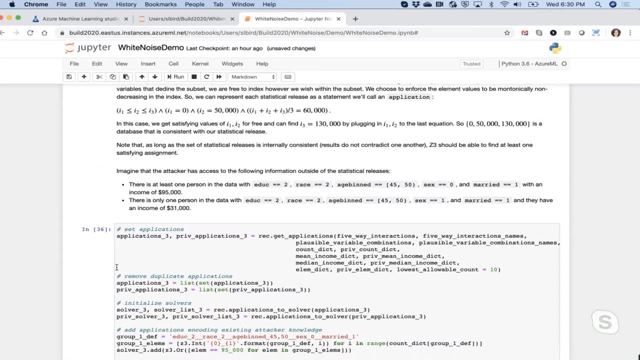 And I want to make sure that I understand. So can you scroll up just a little bit more, Okay, Okay. So, basically what you're doing when you're looking at that formula, you're basically using a SAT solver by filling in information. that's an aggregate. 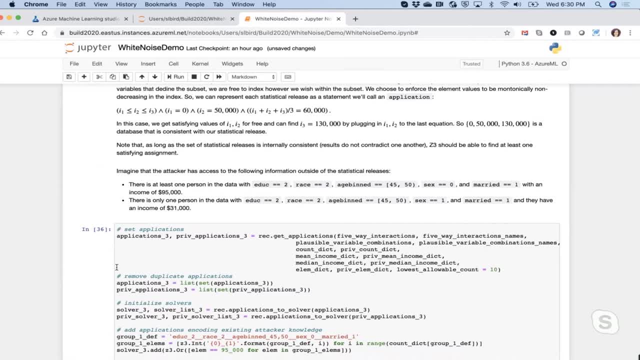 And because you might know a record or two in the database, you can use that SAT solver to reconstruct pretty closely everyone else's income. Am I getting it right? Yeah, For about a third of the individuals. right, we're correctly guessing it. 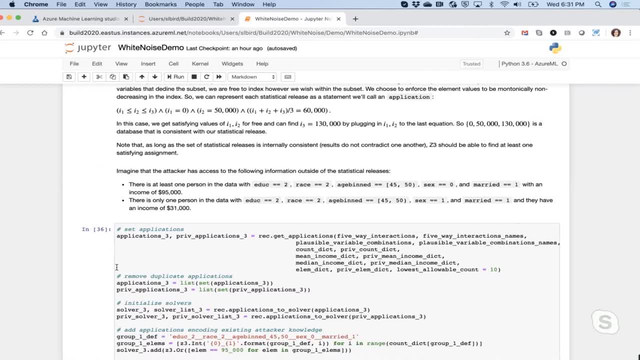 And we wouldn't know which third we were correct for Unless we ran this many times right. If I ran the SAT solver over and over again, I could get a distribution of possible reconstructions and have a much higher chance of guessing the incomes correctly. 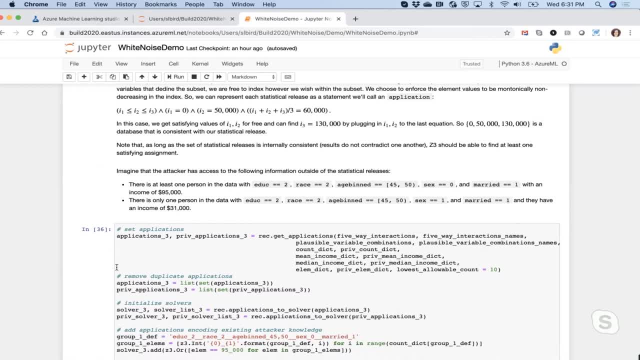 So it's just an example to show how easy it can be to get pretty close on some of this information. And that's surprising to me, primarily because, like let's just say, if you ran it for a day, for sure you could reconstruct it. 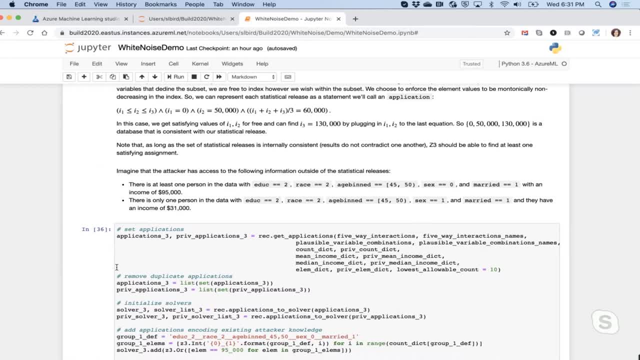 Yeah, And you can see pretty closely what's going on. You're able to extract sensitive information from aggregate data using off-the-shelf stuff. basically, Is that right- And using a little bit of outside knowledge and some other published information- but information that it would be very reasonable to assume is published. 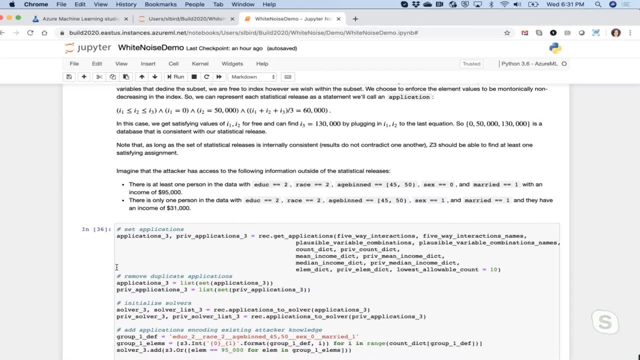 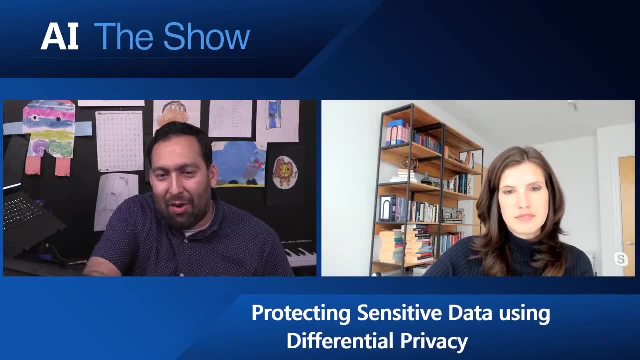 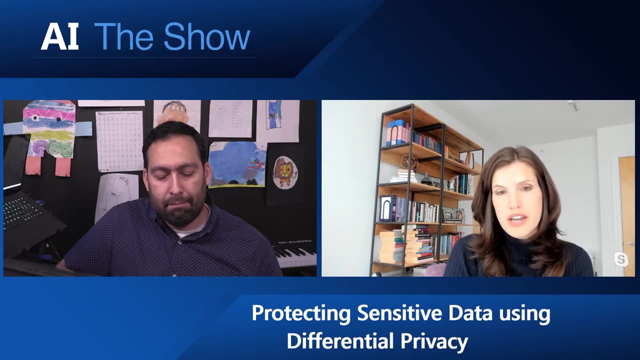 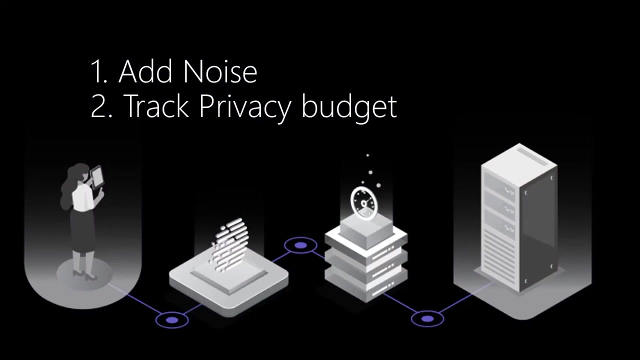 I see. So this is obviously a problem, and there's a lot of data sets out there that may be suffering from that problem. What is differential privacy and how can it help? Is there something we can do to fix this? Yeah, So the way that differential privacy algorithms work is they're actually going to take two steps here in order to mask the contribution of individuals, so that now I won't be able to do this type of attack. 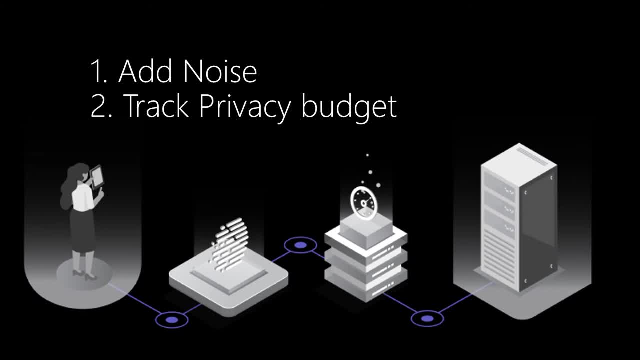 So the first thing that it does is we're going to add noise to that aggregate result. So I can't give you the exact answer anymore. I'm going to give you a list. I'm going to give you the answer with a little bit of statistical noise. 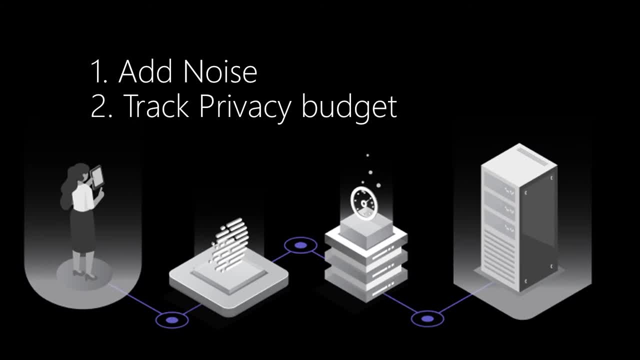 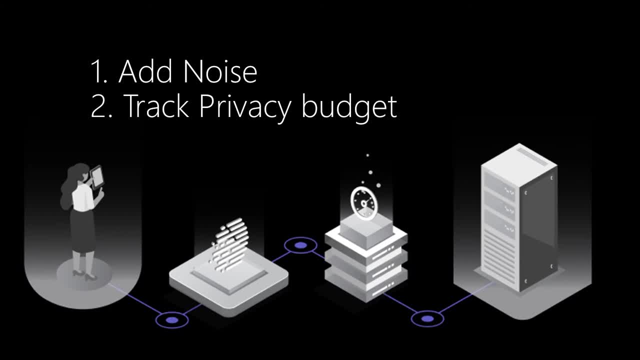 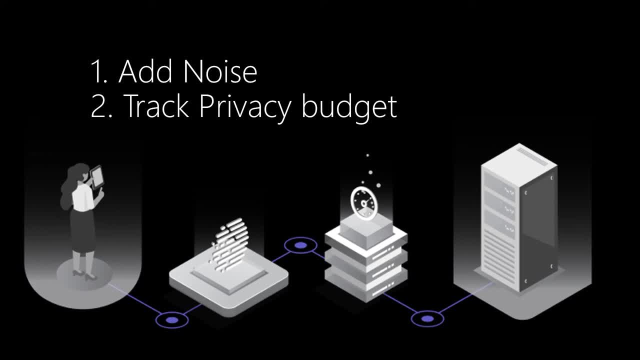 So let me ask you the first question. I saw some of this earlier and it was kind of confusing to me. What we're saying is that are we literally like flipping answers in the database on the add noise step? Is that what's happening? 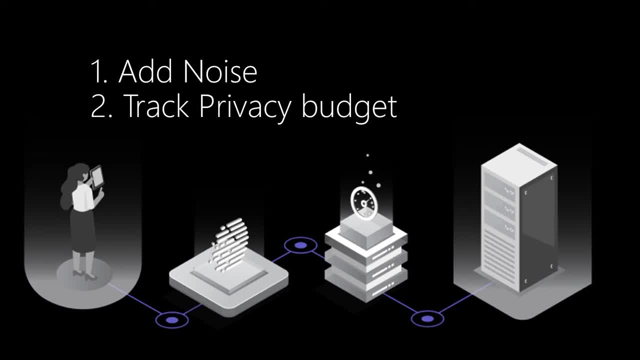 No, It works more. You could think of it as adding a small amount on top of the aggregates. So if my real answer were 60, you might actually give back 61 or 65. So I can actually show you how it works in my notebook. 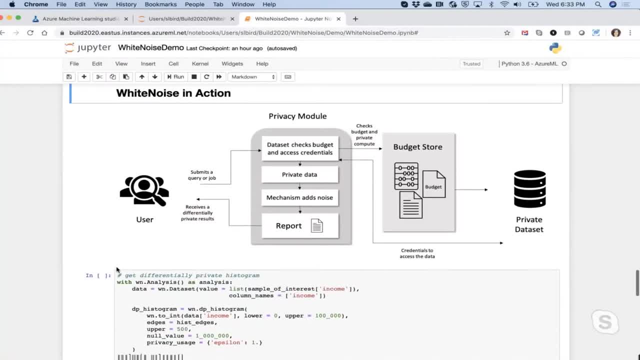 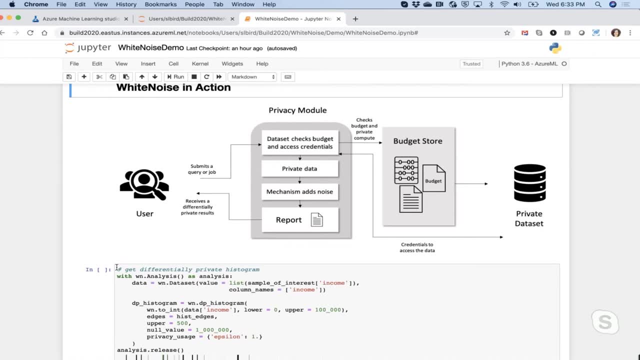 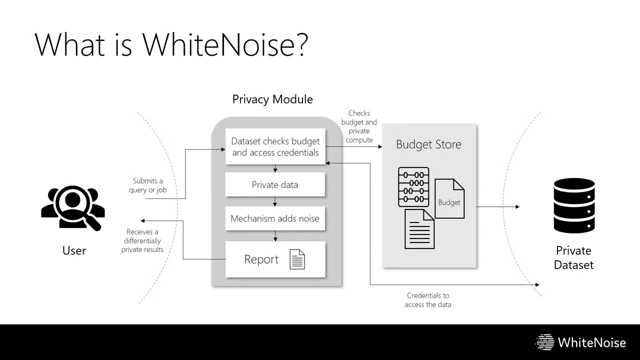 All right, let's do that. So if I move down here, what I'm going to do is now use the white noise system to publish the reports, And white noise is our differential privacy system that we've built, And basically it contains all of the sort of proven differential privacy algorithms that have been developed over the last decade in research. 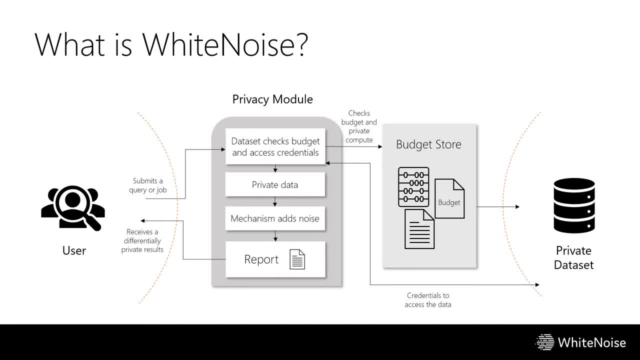 And then the ones that we're finding are actually working well in practice, And so the system sits on top of that data store and does the two steps we were just talking about, So it will take your query. Add that bit of noise, Compute how much information the queries would be revealing. 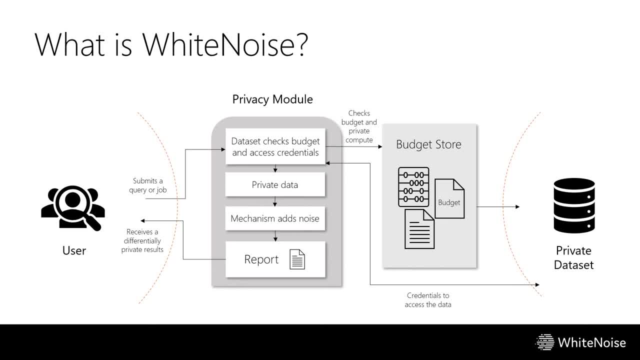 Subtract that from the budget and give your result back. And so now, if I do that here in my notebook, Is it okay if I ask a question or two, Because this is super fascinating to me? So you're saying that the white noise module sits on top of the query? 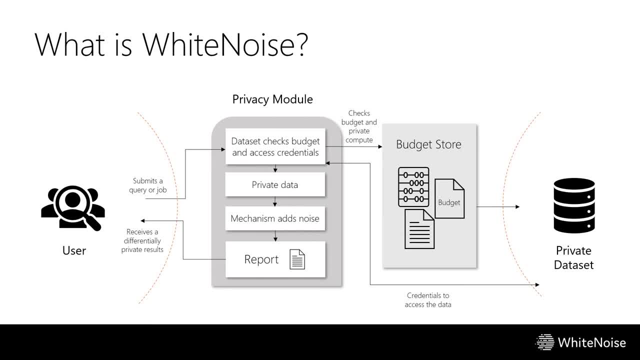 So you're actually querying the privacy module. The privacy module asks the real data for the real aggregate information, And then it adds noise to it in a way that makes the aggregate data still be valid but make it harder to reconstruct original data. Am I getting that right? 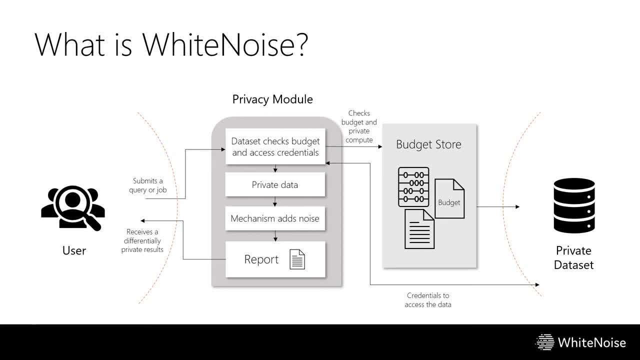 Exactly, Exactly And right now, the system you know we wanted to. you would use it when you have access to the data, But just to guarantee that those reports that you publish or the model that you build has these differential privacy guarantees. 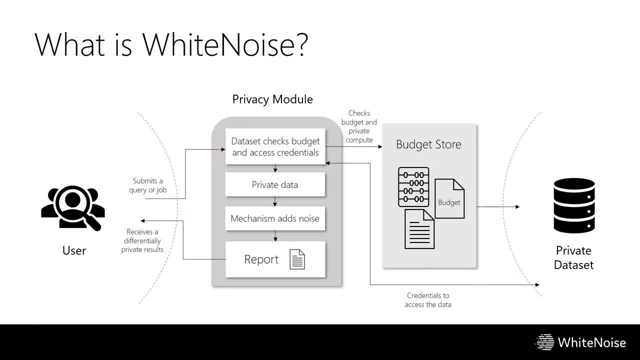 However, in the future, we're also hoping to enable this to be a situation where the data scientist can't access the data set directly, but they could do this query, because it will enable us to allow more people, for example, to do research on top of data sets, do medical research or social science research. 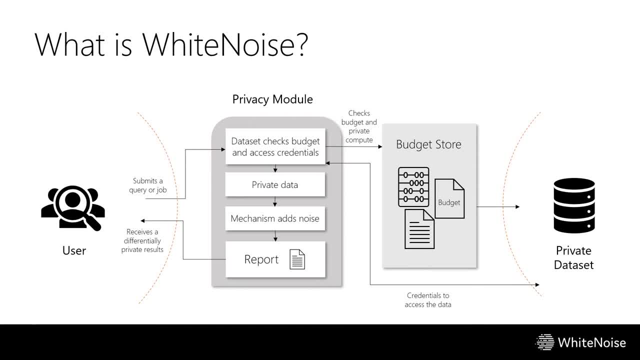 And so we think this is a really exciting direction going forward. Cool. The second question: the budget. And that's an interesting thing because what you're saying is that an attacker knowing, because it's probably some mathematical distributions that you're using to add to noise that are well known- 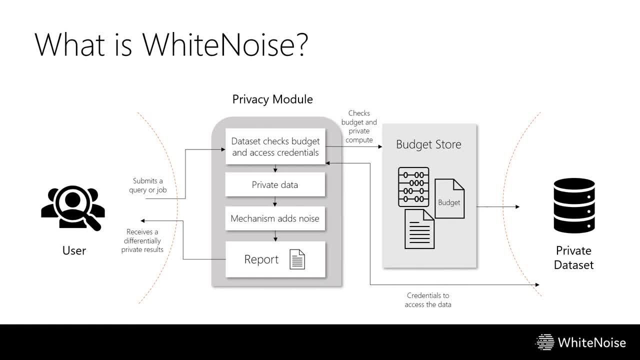 What you're saying is that if the attacker does like really a bunch of systematic queries, knowing the distribution of the noise, they should be able to be able to reconstruct the data. And so the budget is just saying you can only query this so many times. 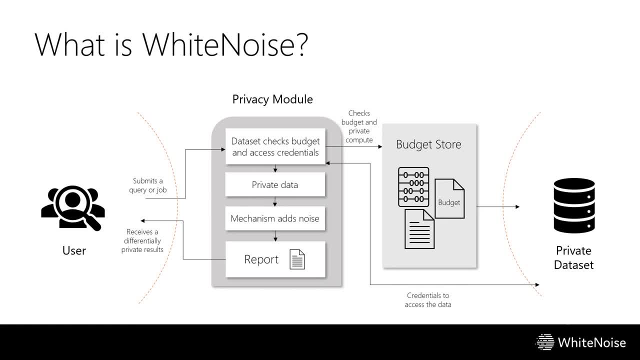 Am I right on that? Because that's what I'm getting, but I want to make sure I'm correct. Yeah, I think it's basically that if I reveal too much information, then you could basically remove the noise. right, You could understand what the noise that was added is. 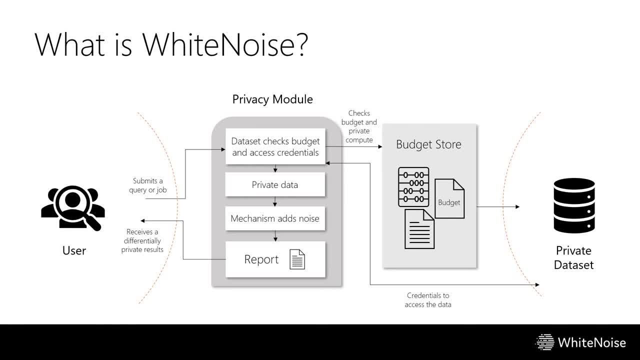 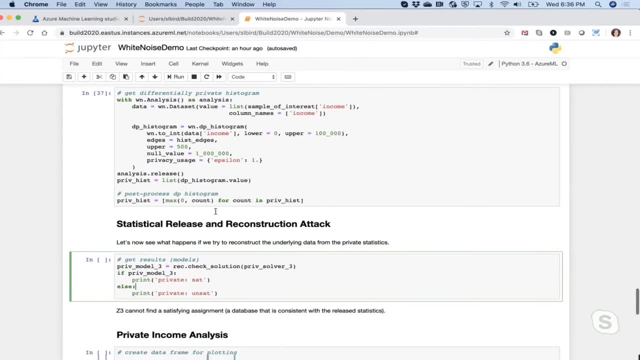 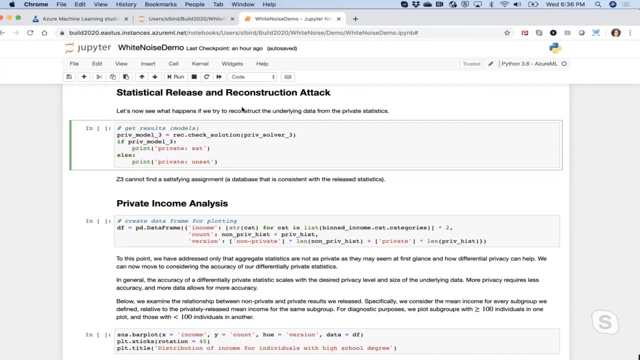 And so you could get that private information. All right, Well, let's take a look at the demo. Great, So I use the white noise system above here to generate some histograms, And then what I'm doing now is I'm first going to show that we're achieving what we said we would, which is not allowing that type of attack. 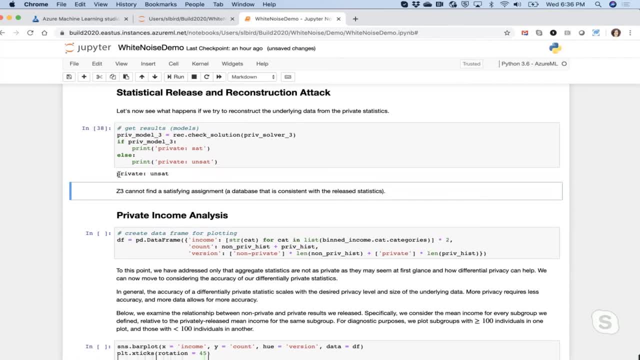 So I'm going to do the same: SAT solver, But what we get back now is unsat, which means it couldn't find a database that said it satisfies the output, the reports that were published, So it doesn't have any guesses in terms of people's income, which is great. 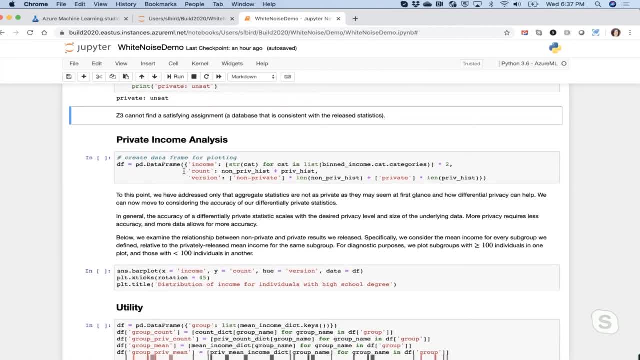 So we've achieved one goal here, But we also need to show that the data is still useful. right, We're adding noise, And so people often ask: well, what am I going to do with noisy data? Right, How useful is this? 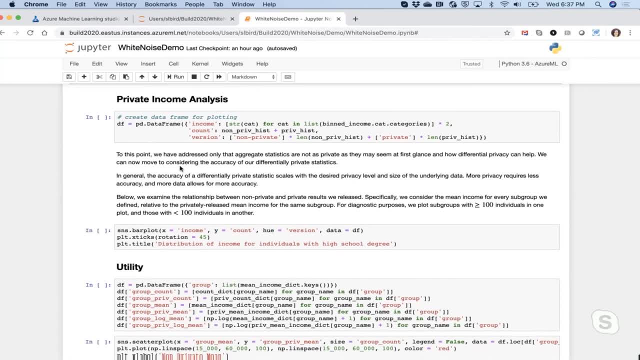 And so I still want to be able to do that private. I still want to be able to do that Income analysis, But now we're going to do it using the private data, And so, if I generate my plot here, here are the two results side by side. 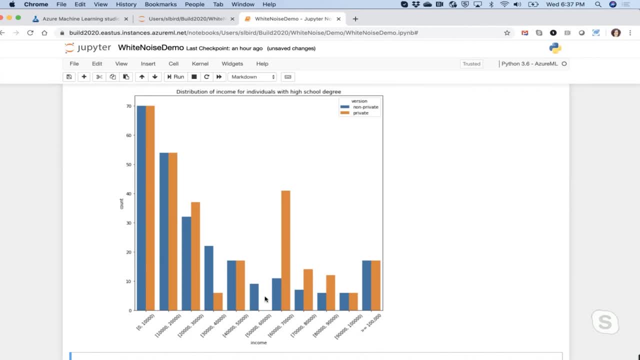 I have my non-private version, which we saw above, in blue and I have my private version in orange, And what we see here is that in some cases it's actually quite close Right. A very usable noise is very small. In other cases, the noise is actually quite significant. 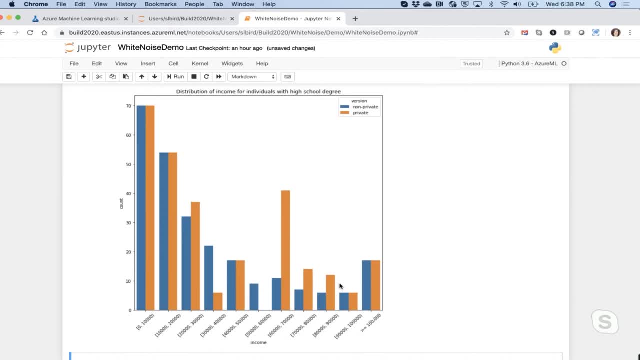 But and that's because these are really small values And so the relative noise we're adding could be a lot more, And so it depends how. for how usable it is, It's going to depend on, basically, how large your data set is and how much noise needs to be added, depending on what privacy you need. 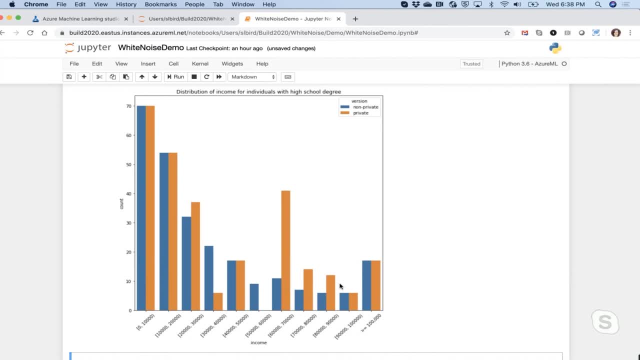 But if you're using- in this case we're using- a pretty small data set so that I could show the attack in my notebook, But If you're using a very large data set, which is the case for a lot of our machine learning and statistics, then the amount of noise that's added is often negligible. 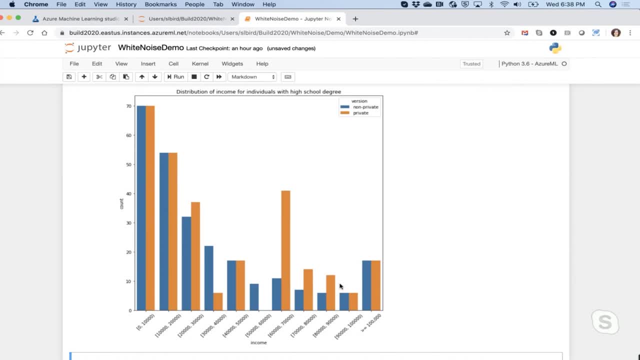 So, looking at this, my guess is that there is some kind of slider between how much privacy you want and how much noise is added. Is that an accurate statement? Yeah, exactly. And and how much budget you want to spend on a particular query. 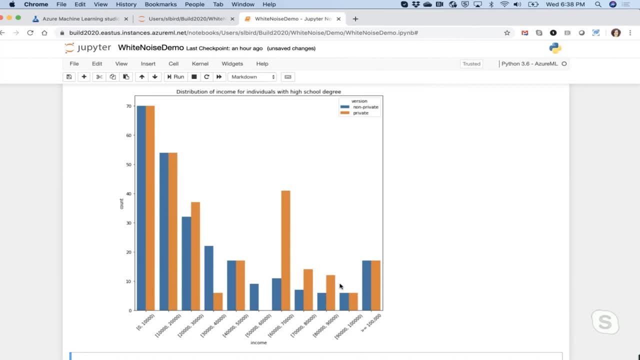 Right, If I'm willing to spend, if I only want to do one query and I'm willing to spend all My budget on that, I can get a lot more accurate information than if I want to do many different queries and I only want to use a little bit of budget on each query. 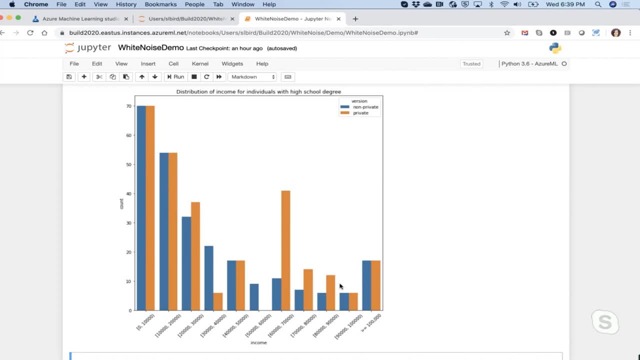 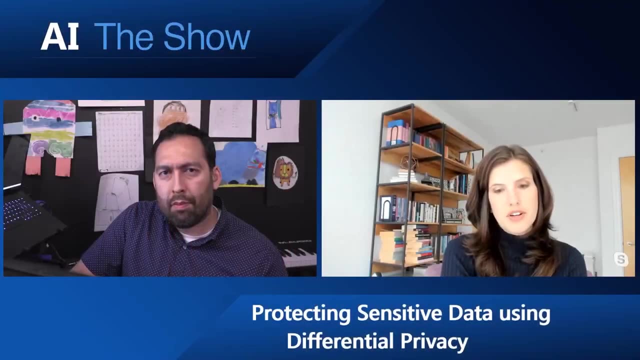 And then, of course, how- how private you want it to be affects the accuracy, And then, as I was saying before, the scale. So if it's a very large data set, you'll still have that slider, but it'll look much lower in terms of the tradeoffs. 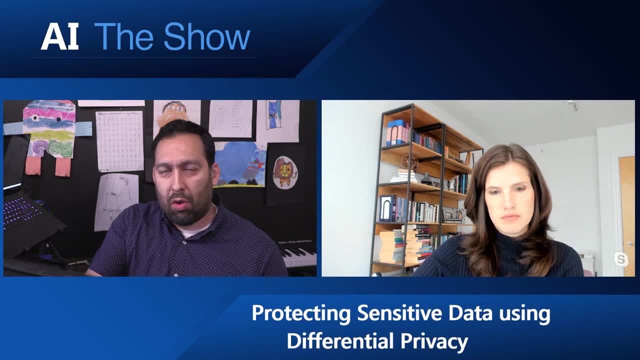 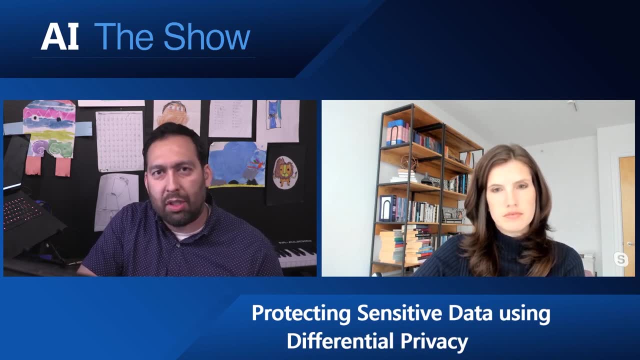 I see. So basically you're putting the user in control over How private they want the data to be, how big the budget is, et cetera. It's all a user kind of approach to this. Yes, absolutely Fantastic.